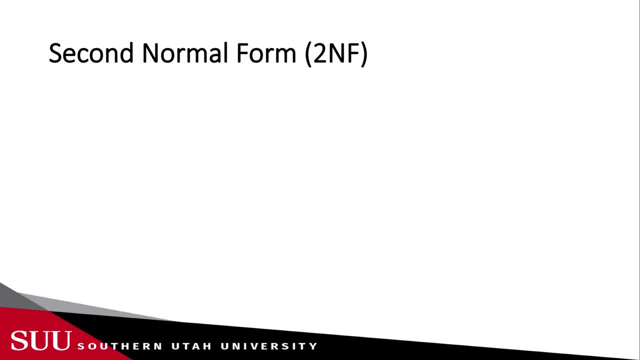 is the second normal form. Let's see what are the rules of the second normal form. It says the second normal form is nothing but the first normal form, but we need to remove any partial details. So the main rule of the second normal form is to have the first normal form. 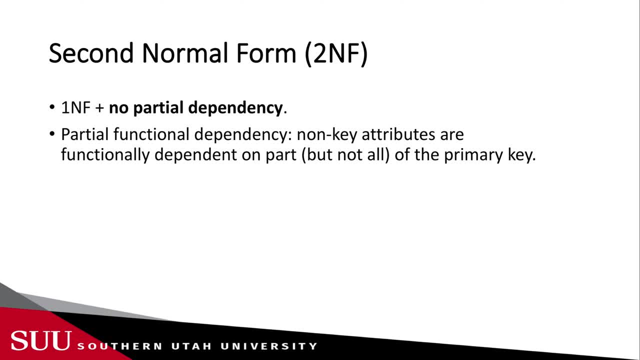 and its Integral Key Elements. Now the main rule of the second normal form is having a Partial Dependency. so a partial dependency again is defined by when the non-key attributes are functionally dependent on a part, but not all, of the primary key. So every non-key attribute must be defined by the entire key, not by 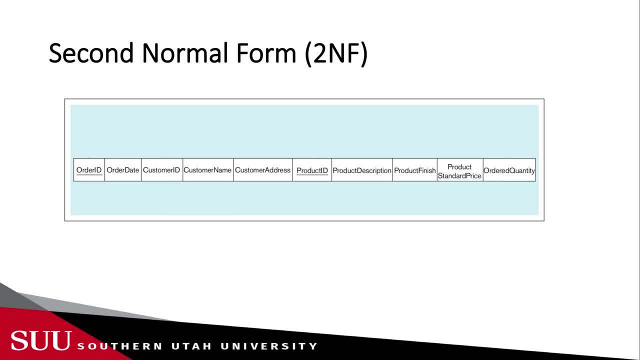 look at the table that we just had. we don't need the data because we just need to define the dependencies. in this case, what sort of partial dependencies do we have in this case? so, if we look at order ID, will have order date and we will have. 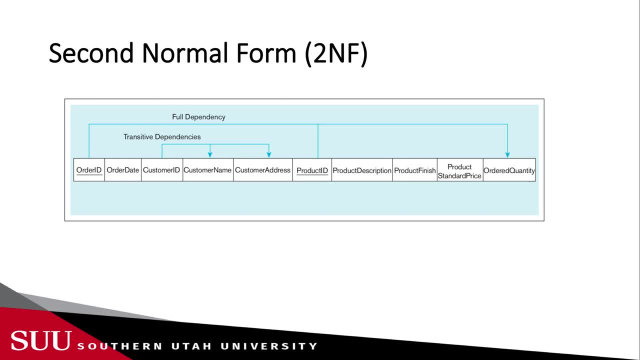 customer ID will have customer name. so we will have many dependencies in here. so on order ID will have order ID, customer ID, customer name, customer address, depending on just one part of the key. and then we will have another partial dependency on product, which is product description, finish and center. 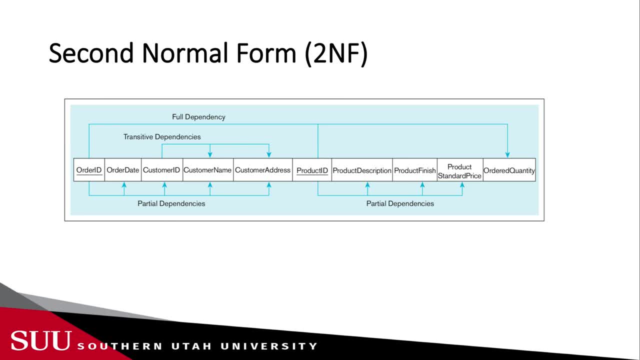 price, all relying on product alone. we also have some other dependencies, which are transitive dependencies that we'll talk about later on, but we also have a full dependency, which is good. so we have a full dependency, which is order ID, product ID and quantity ordered. so we 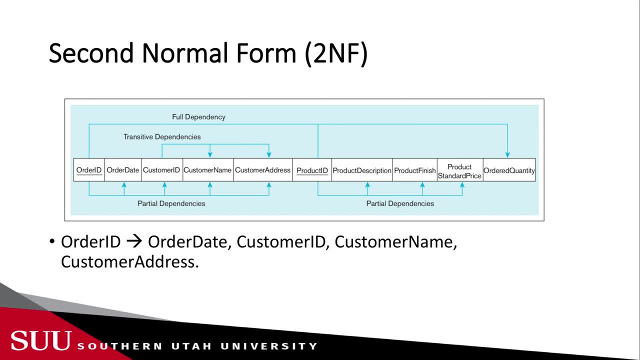 need to remove the partial dependencies to get into the second, normal form. so we define our dependencies. these are all the dependencies that I have, so I defined all of them. you can see that I have all the dependencies that I have, so I defined all of them. but then we only care about partial dependencies. so how do we remove them? we? 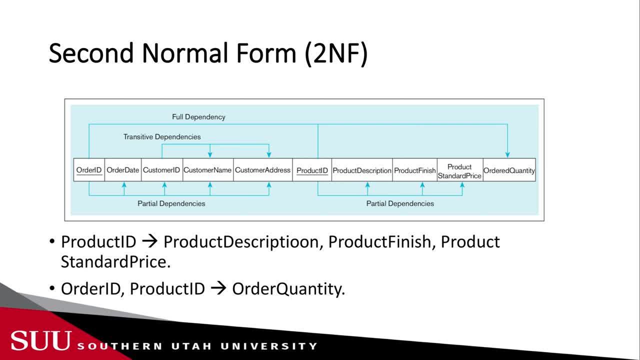 need to make them full dependencies. how do they become full dependencies if they are in their own table? so we need to make those partial dependencies full dependencies. we we already have one full dependency, which is order ID, product ID and then quantity order. so this is going to 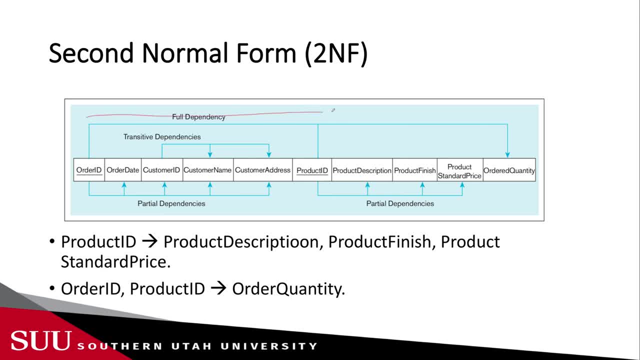 become one table. so this full dependency is going to become one table, containing one, two, three attributes, and then each one of those partial dependencies is going to have its own table. so this is going to be a table and this is going to be another table as well. 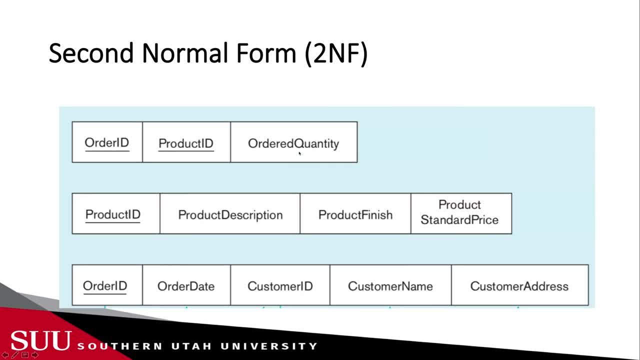 so the resulting second normal form is going to be what we have in here. so what we did is we made the partial dependencies become full dependencies by separating them in their own tables. and now, if we look in any one of those tables, we do not have any partial dependencies. now what is next next? we 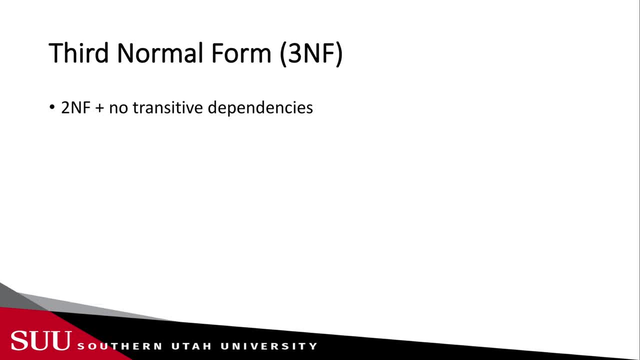 come up to the third normal form. so the third normal form is when we have the second normal form. we just need to remove the transitive dependency. we just seen the transitive dependency in the dependency in the previous example, but we will define it now and then we'll visit it again. now our transitive dependency is a. 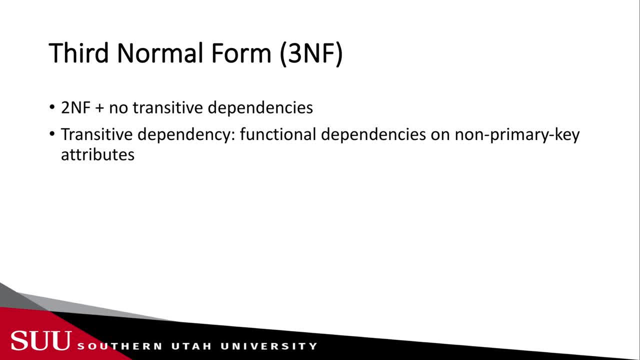 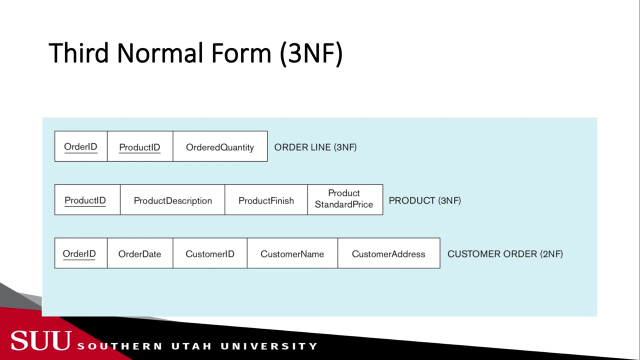 type of functional dependency on the non primary key attribute. so the solution, the non key determinant with transitive dependency go into a new table and the non key determinant becomes the primary key of that new table and stays as a foreign in the old table. so if we look back at what we had, we had the second normal form and 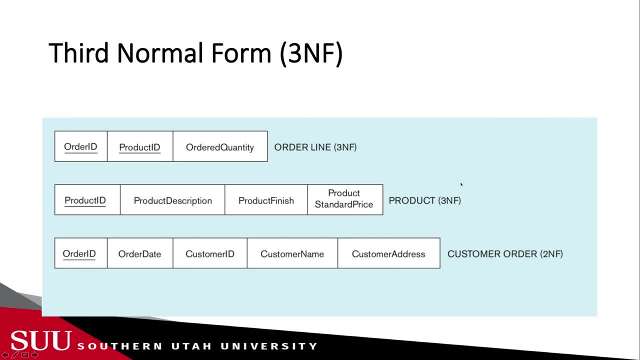 if we look closely, this is already in third normal form. this is already in third normal form, but this is in the second normal form from the previous step. now why is it in the second normal form? the thing is: customer name and customer address will rely on the customer.